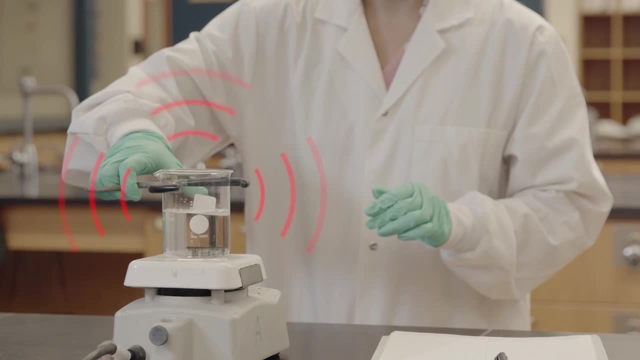 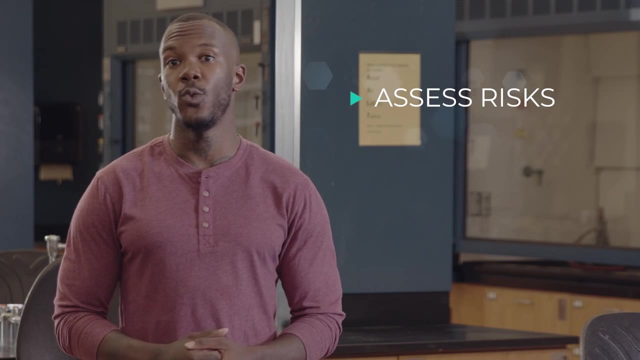 If a solution needs to be heated, the source of heat creates the hazard. This is especially true if one of the chemical reagents is flammable. Step two of RAMP is about assessing risk. Risk is the chance of being harmed by a hazard. 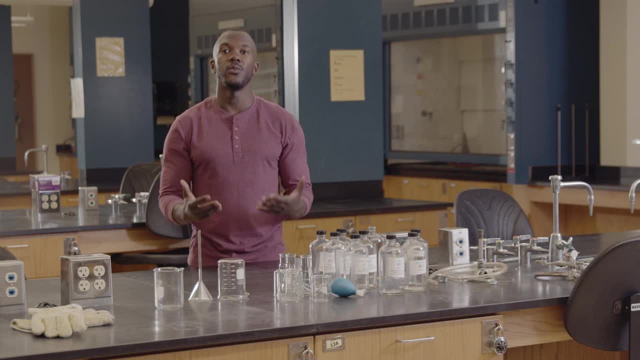 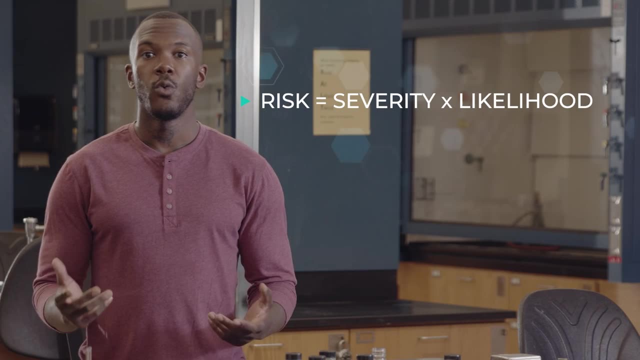 Even if a chemical is hazardous, it doesn't necessarily present a significant risk. Risk is a combination of both the severity of hazard and the likelihood of exposure. You can think of it like this: Risk equals severity of hazard times the likelihood of exposure. 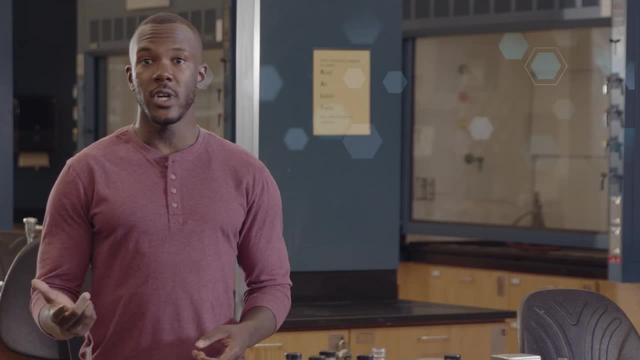 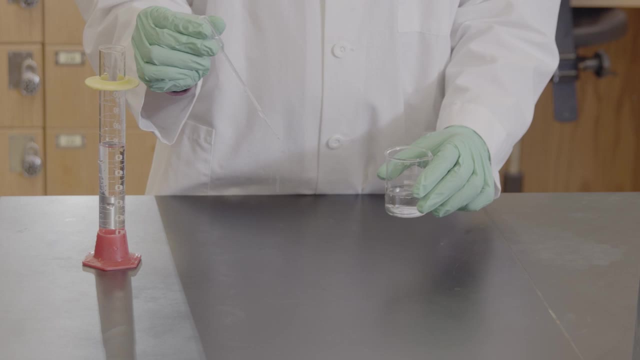 For example, a solution with a high concentration of nitric acid is very hazardous, since it is both a strong acid and a good oxidizing agent. It's easy to control one drop, And if it got on your skin, it could be easily washed off. 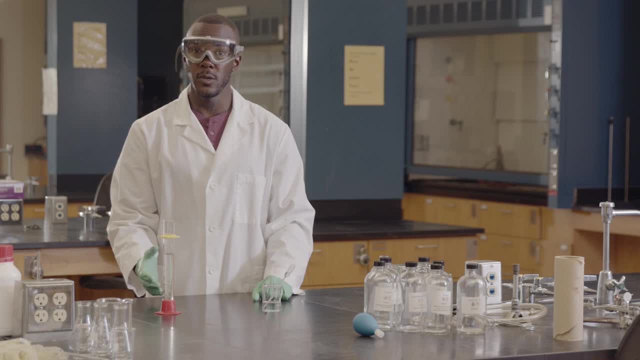 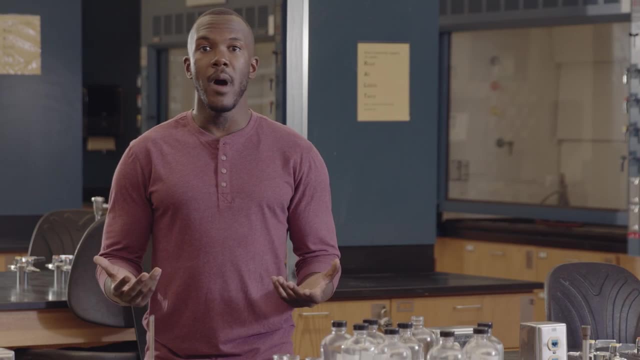 On the other hand, if you spill 50 milliliters of the solution on your leg, you get a lot of exposure and it could cause significant damage. You can see that the amount of the acid and the way it's used affects the level of risk. 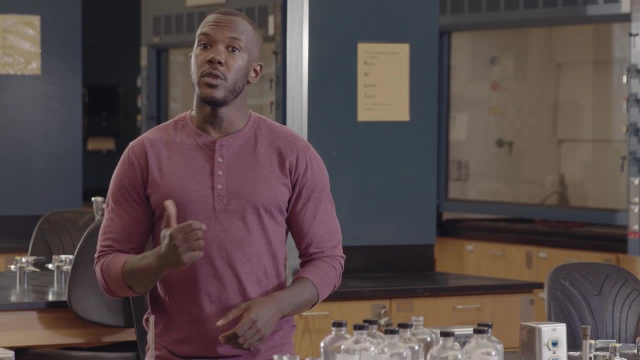 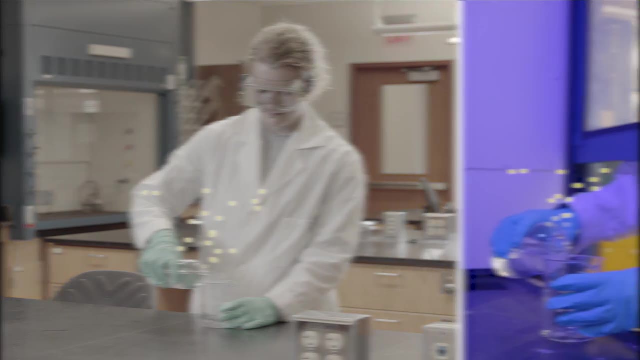 Another example would be the use of a liquid like ethyl ether, where the vapor is unsafe to breathe. Using this in the open part of the lab presents significant risk. Using it in a chemical hood is much safer, since the likelihood of inhalation is greatly reduced. 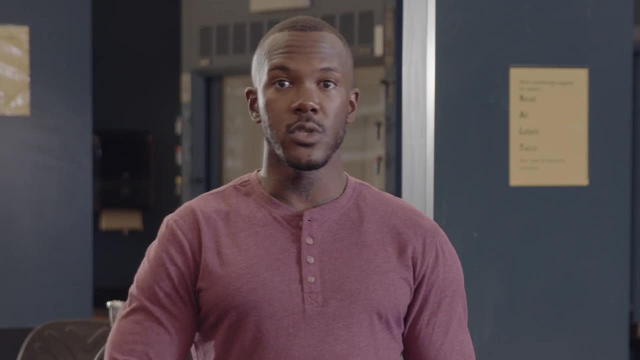 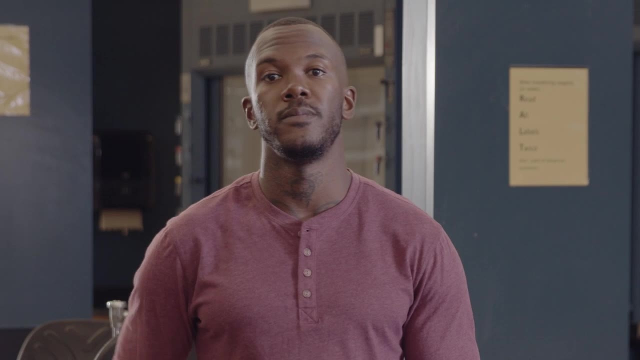 We'll dig deeper into assessing risk in another video, but for now just remember: all experiments pose some risk and most experiments can be done safely if the risk is reduced to acceptable levels. The third step in RAMP is to minimize risk from the hazards. 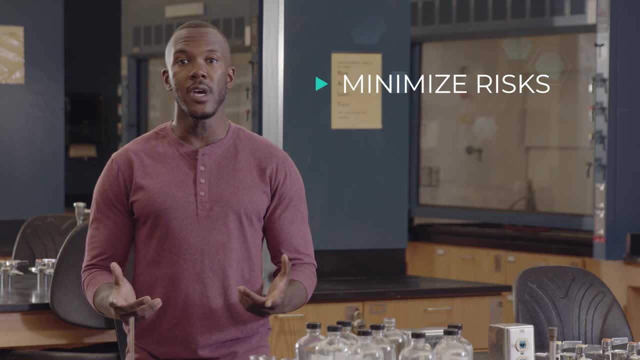 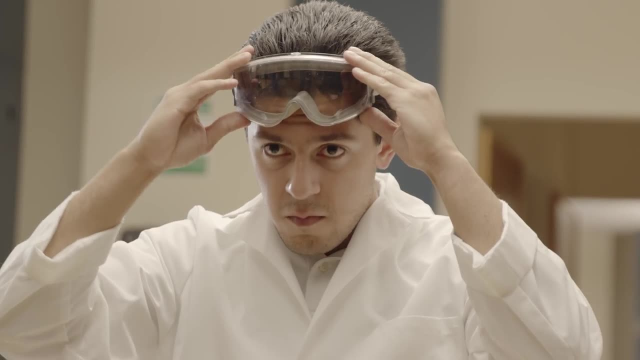 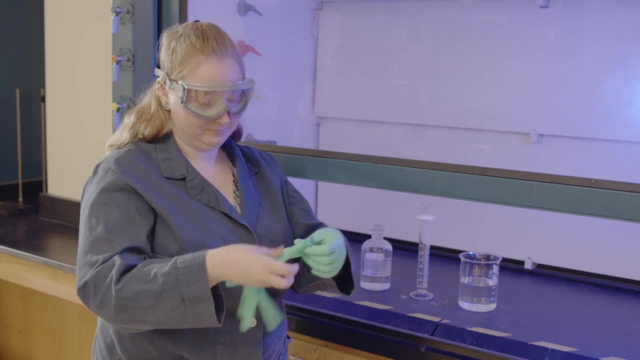 This is the origin of many familiar lab rules: For example, working in a chemical hood to avoid breathing hazardous gases and vapors. wearing eye protection to avoid any possibility of corrosive substances damaging sensitive eye tissue, and wearing gloves and or a lab coat when a procedure may expose skin to potential injury. 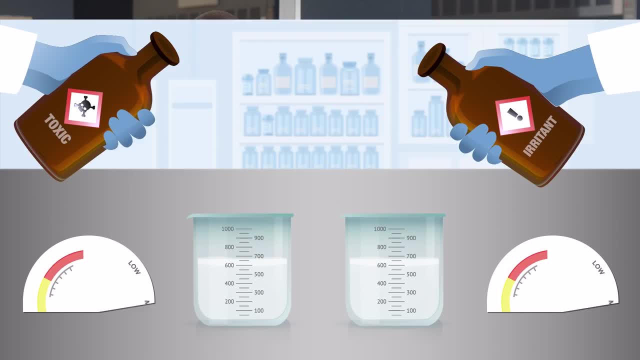 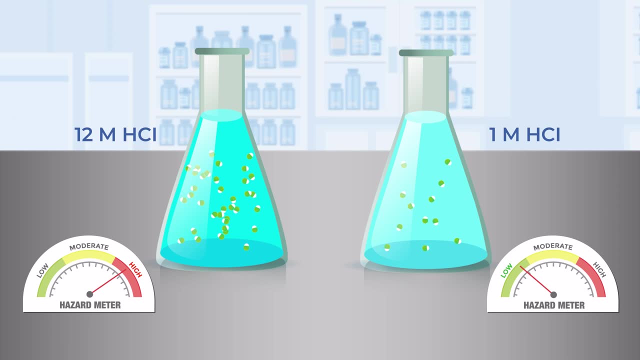 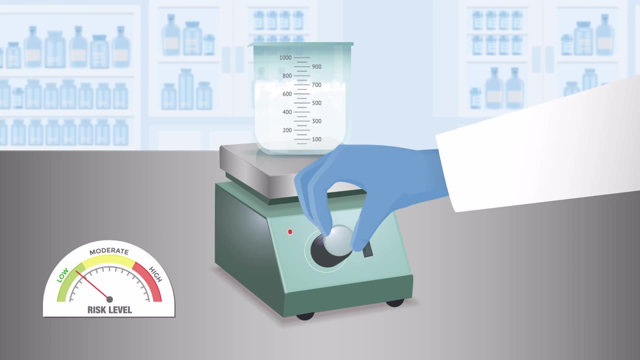 Here are some other questions you can ask to help minimize exposure. Can you use a less hazardous chemical in place of a more hazardous one? Can you use lower concentrations of chemicals? Can you run a reaction with smaller amounts of chemicals? Can you lower the temperature to reduce the risk of burns?